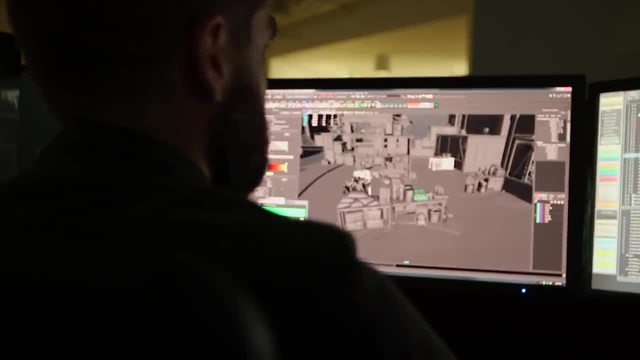 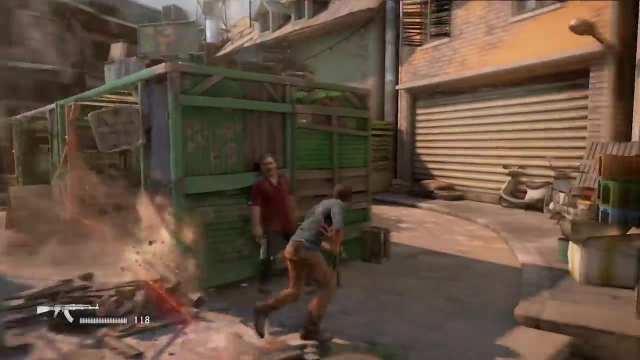 very necessary role for all projects, no matter what your field is. They are tasked to create a wide range of elements and objects, such as weapons, vehicles, furniture and so on. Basically, they create all the props for video games, movies and animations. 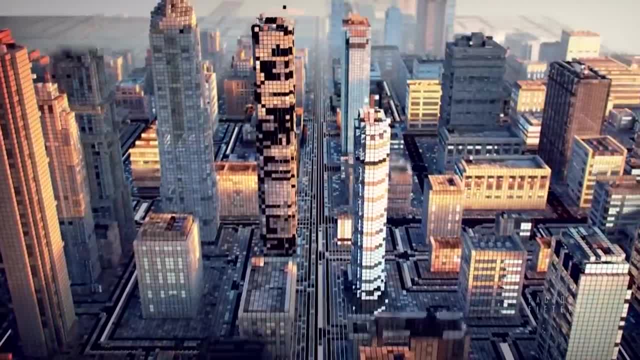 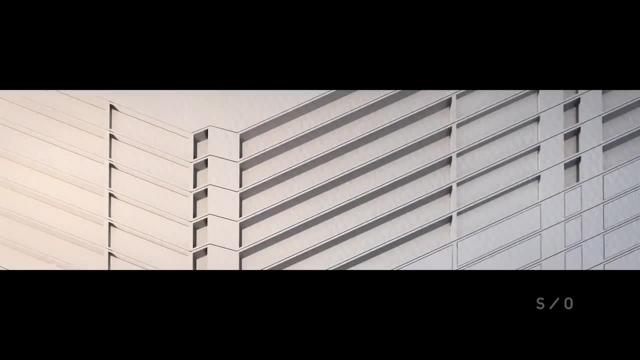 This is quite a fun job for those interested, as 3D artists, or specifically, visualization artists, work closely with architects, meaning that artists will be interpreting the blueprints and designs of construction, in addition to houses and interior designs, and try to bring 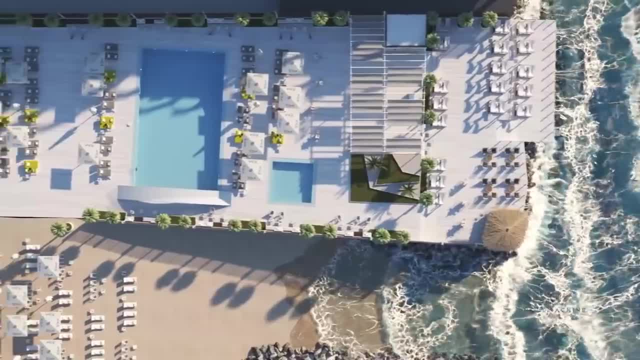 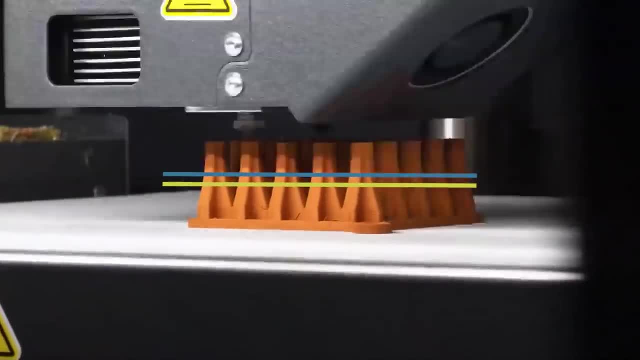 the architect's idea to life, all for the sake of tackling, simplifying and visualizing plans to the clients prior to the actual execution and construction. 3D printing is relatively a new field. and it is a relatively new field, The 3D printing. 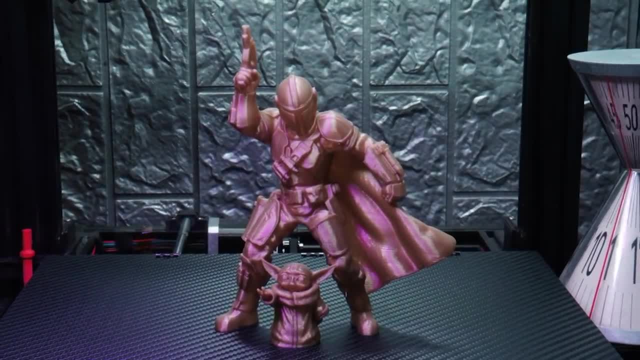 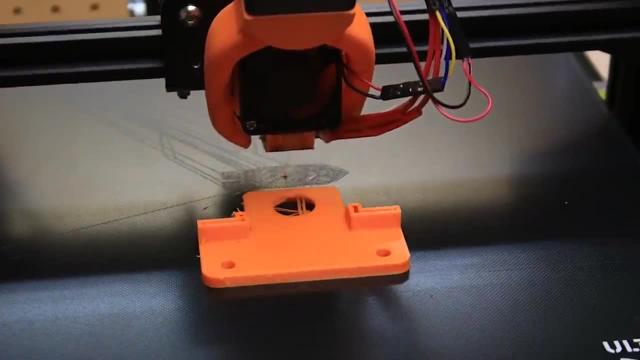 field is a growing industry, as 3D printing companies are everywhere to offer a variety of printing services for clients. What is the task of a 3D modeler, you might ask? Well, these companies recruit 3D modelers to create 3D models and sort of maneuver the printers. 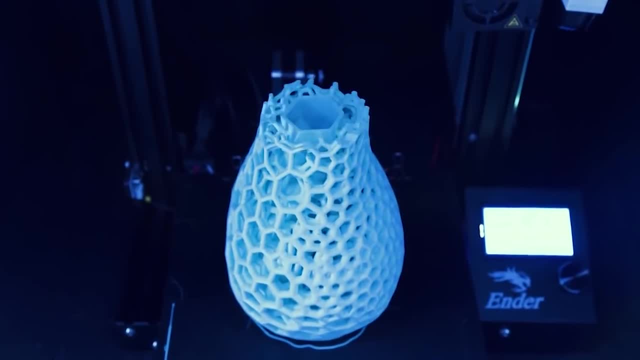 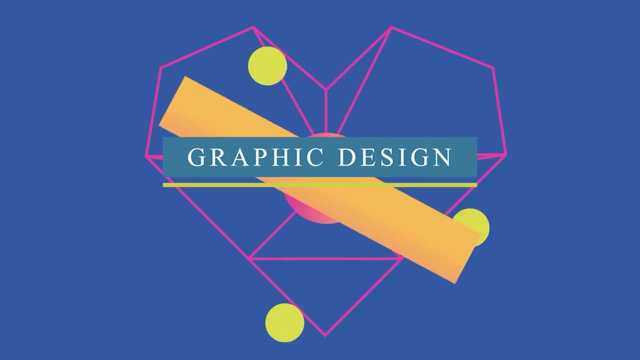 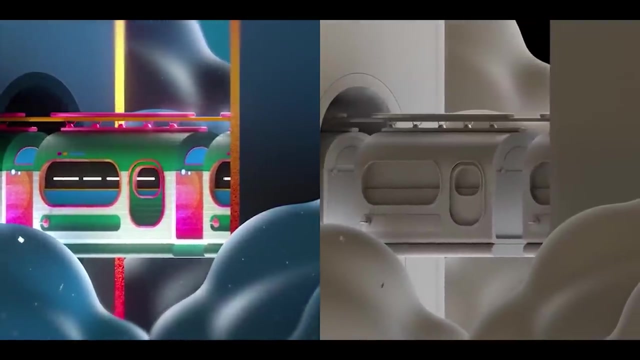 by adjusting and optimizing 3D products and objects for the machines and deliver great 3D printed projects at the end. Graphic design has also been a heavily in-demand profession and the implementation of 3D in it is becoming more intensive. Graphic 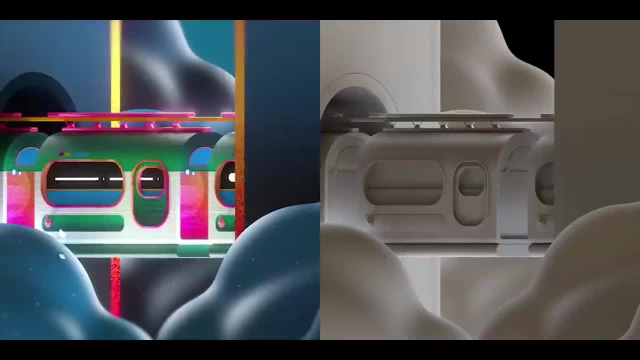 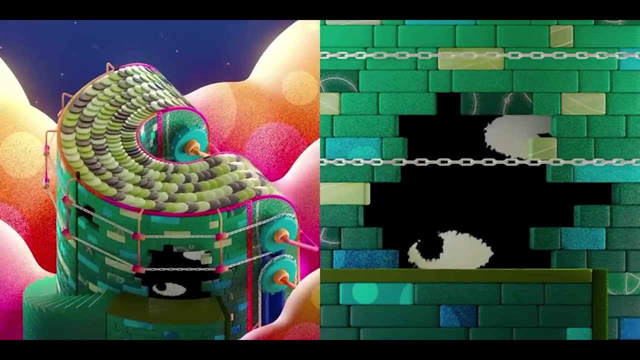 design companies are, frankly, all over the place, which increases the need for 3D modelers. 3D artists often create different kinds of models and create animations for companies and clients to bring their vision to life and help them achieve their goals. So if you 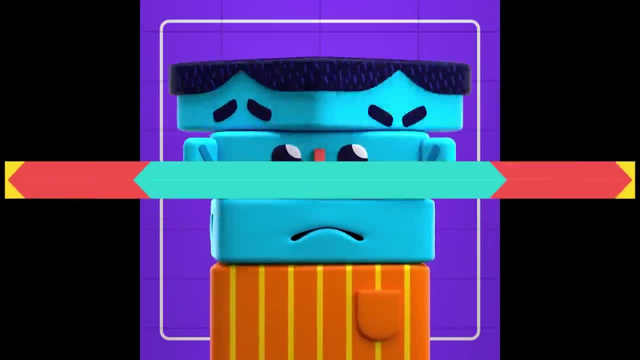